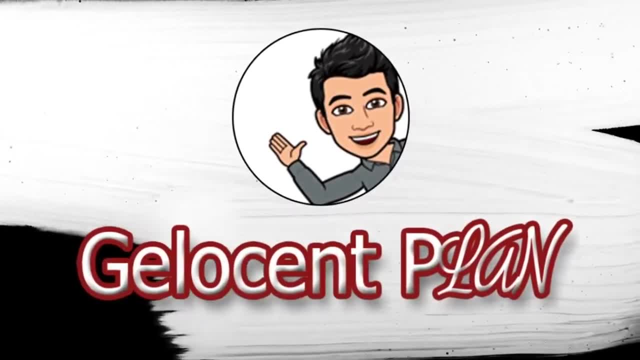 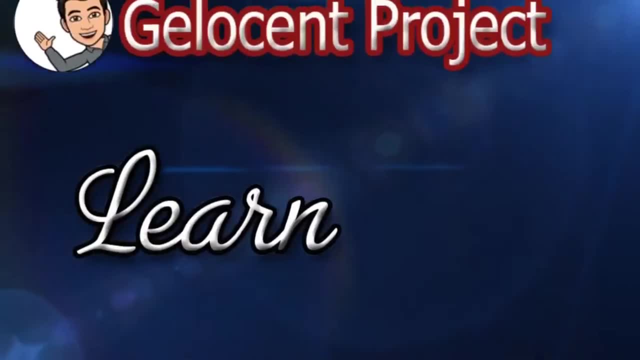 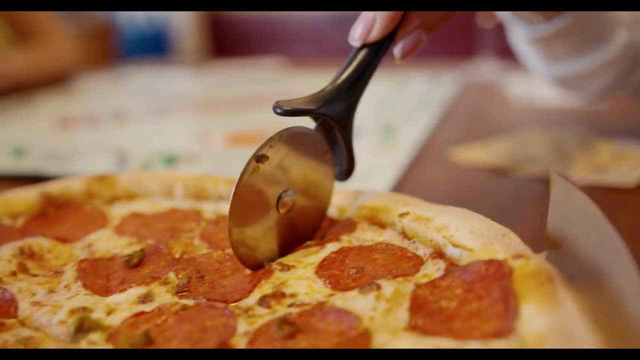 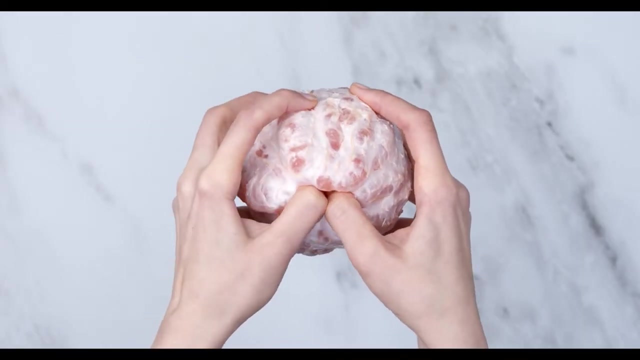 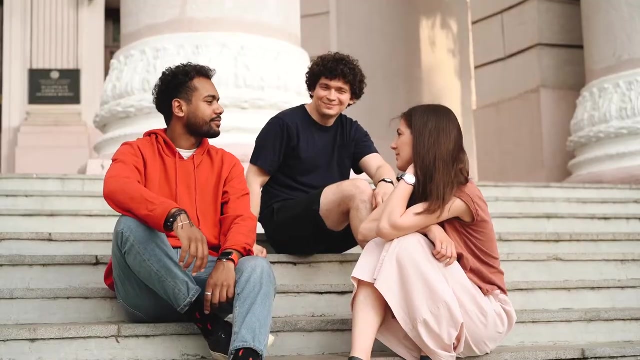 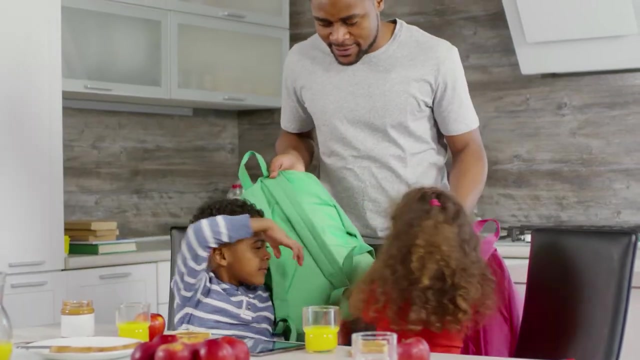 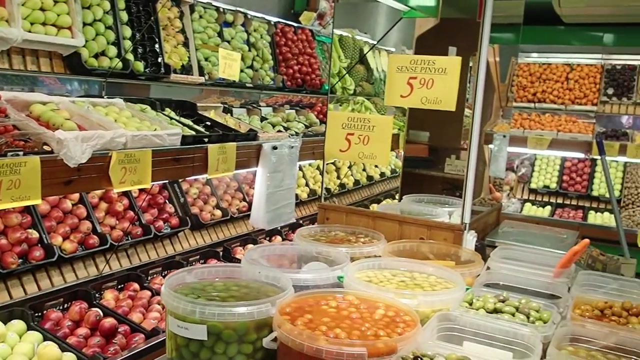 You slice a pizza, You slice a cake, You divide your fruit because you want to share. Sharing is a great thing to do: Sharing it to your friends or sharing to your loved ones. You even go to the market to buy. what you want to share, You also buy. 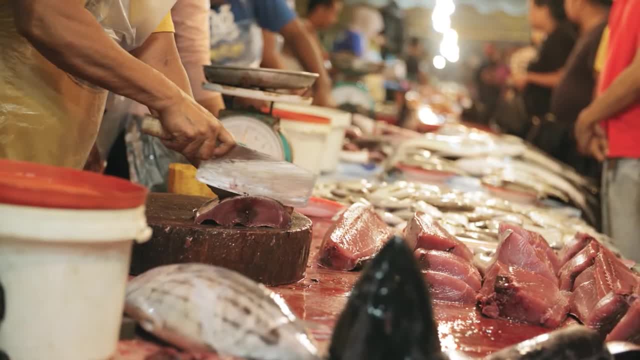 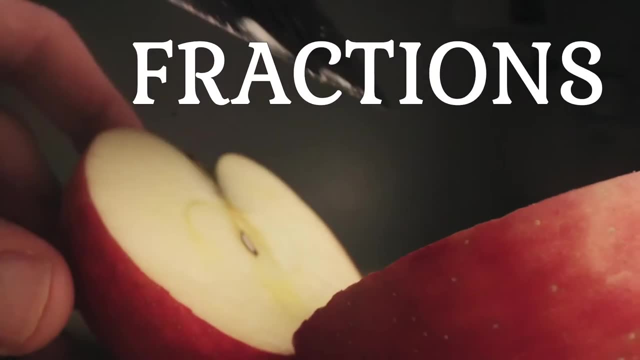 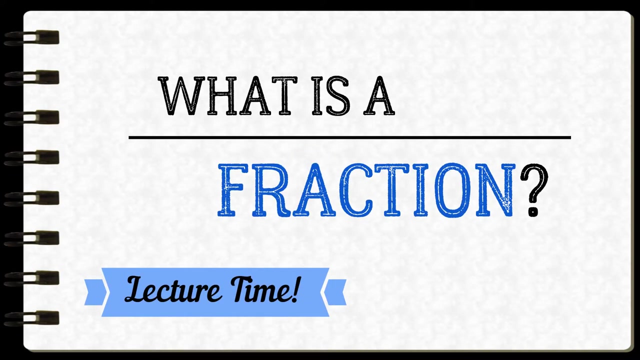 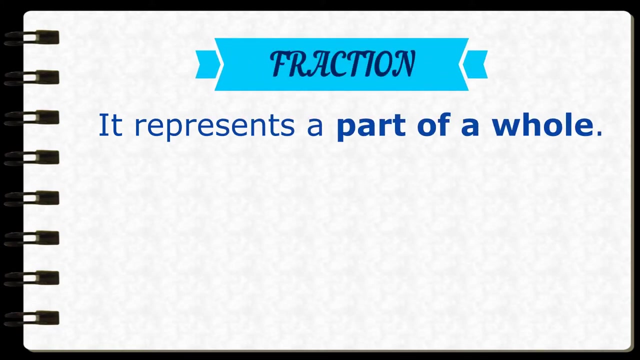 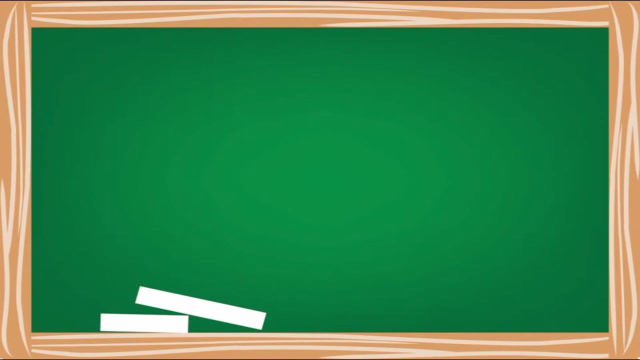 a certain part or amount of food. These are some of the real-world facts about fractions. So what is a fraction? A fraction represents a part of a whole. It is usually written with a numerator and a denominator. Let's have an example. Let's say two-thirds. 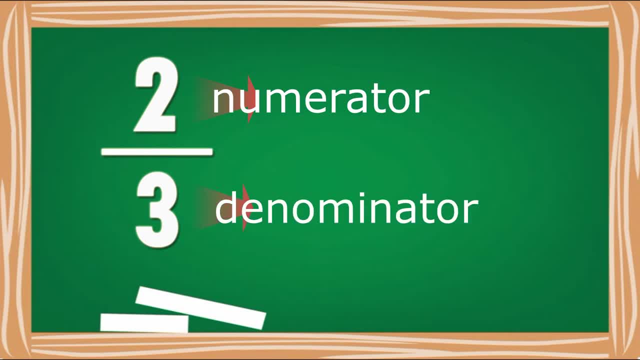 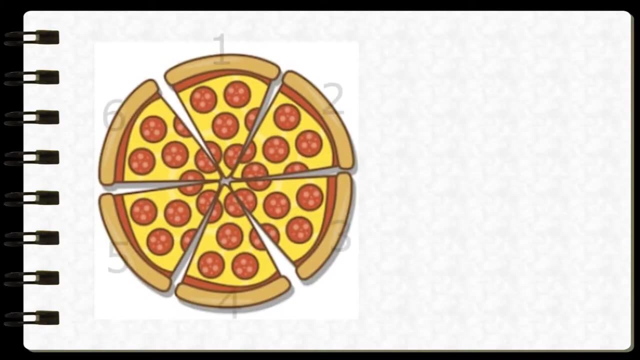 Two is called the numerator, Three is the denominator. The line between them is called the fraction bar. Now, to understand it, let's slice a pizza. How many slices do we have? So there are six slices. The number of slices we made to the. 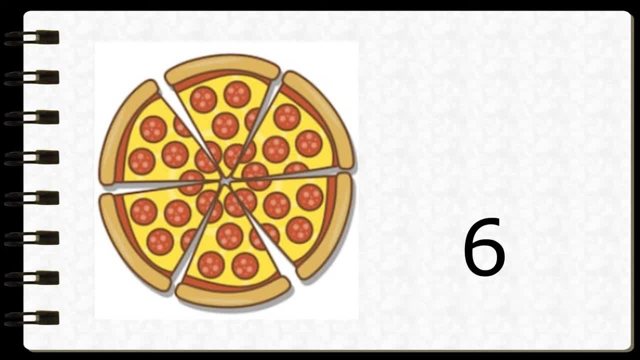 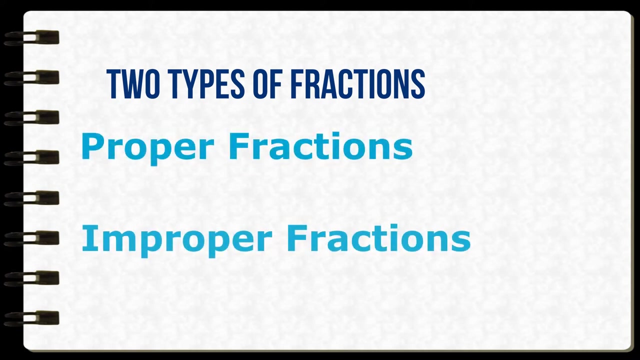 whole pizza represents the denominator. Now you eat one of the slices. The number of slices you eat represents the numerator. Hence the fraction of the pizza you eat is one out of six or one-sixth. So basically, there are two types of fractions: Proper and improper fractions. Can you guess? 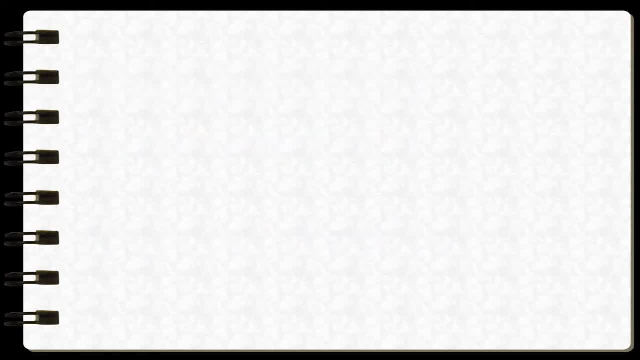 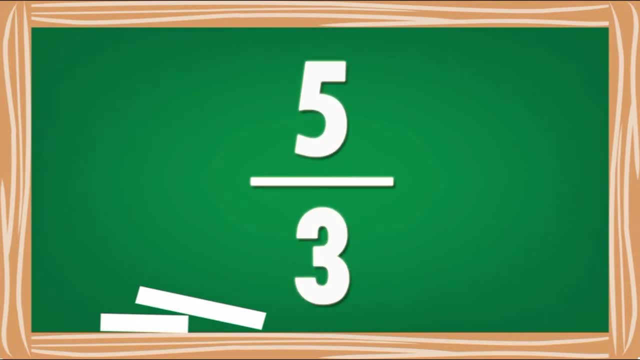 which fraction is proper and improper. Two-thirds Proper fraction. Five-thirds Improper fraction. Nine-fifths Improper fraction. One-sixth Proper fraction. Eight over seven Improper fraction. Three-fourths Proper fraction.